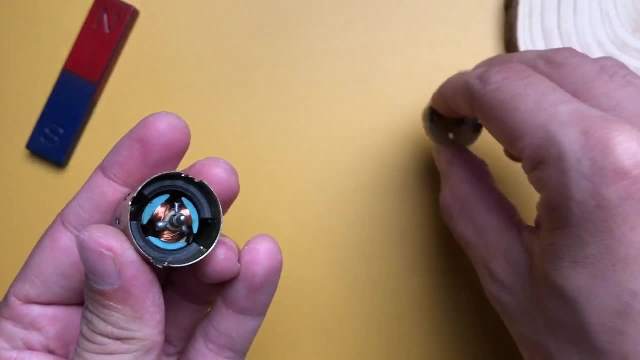 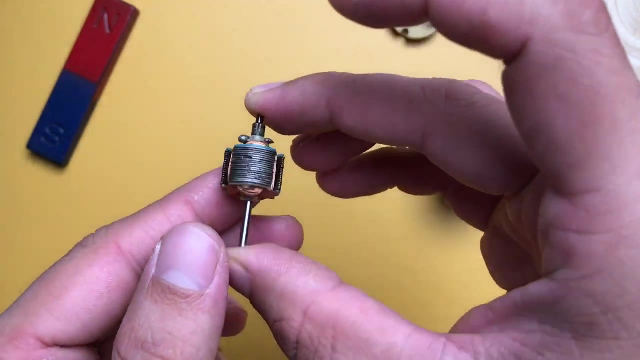 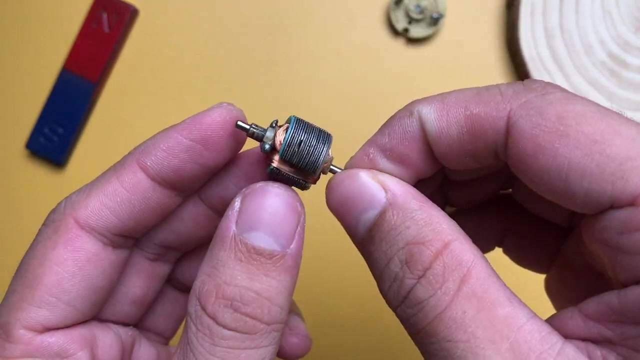 DC machines are one of the fantastic creations we have, Of course, because of the superior characteristics they offer over other machines. Studying DC machines very clearly also helps in creating a very strong base for transformers and induction motors. In this course, you will not only understand both DC generator and DC motor. 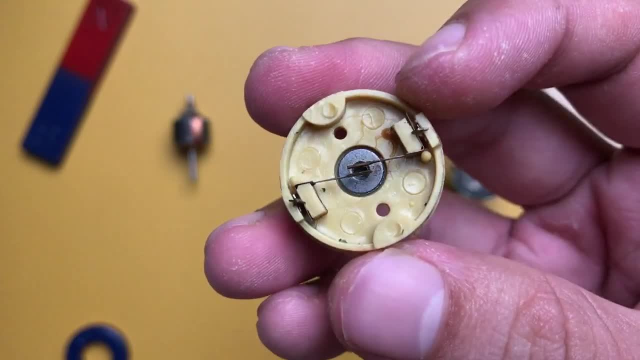 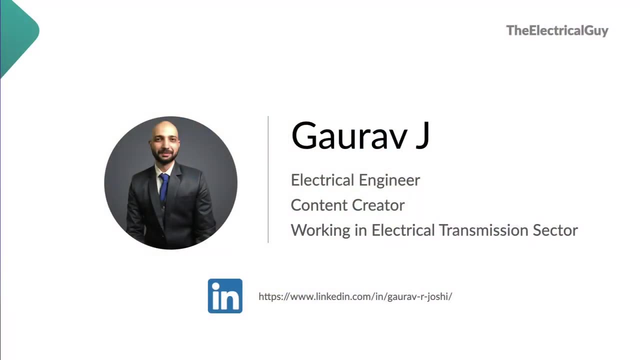 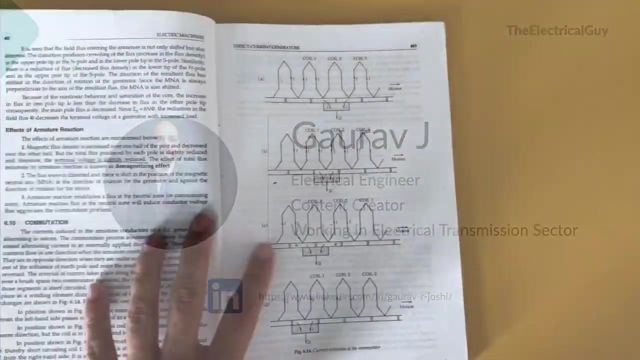 in a very systematic and easiest way. but also, you will be developing interest in electrical machines. Hello, my name is Gaurav J. I am an electrical engineer and a content creator and currently working in the transmission sector- for more than 5 years now, If you notice. 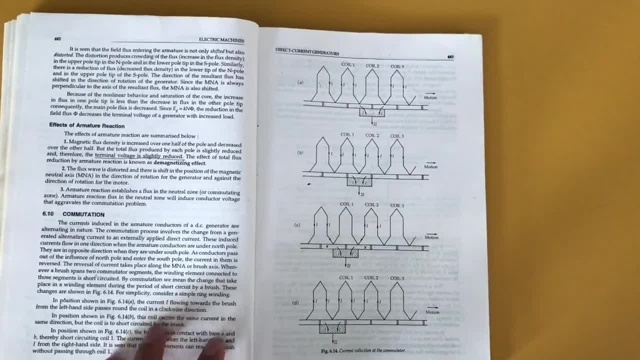 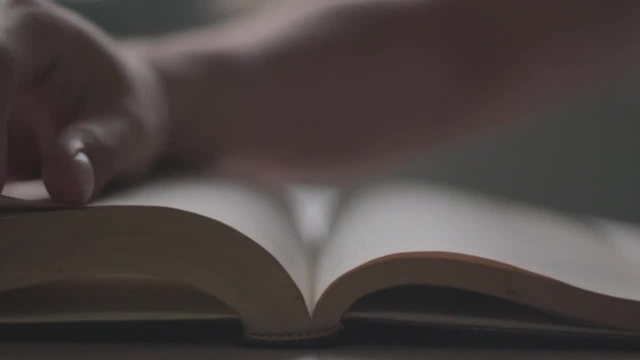 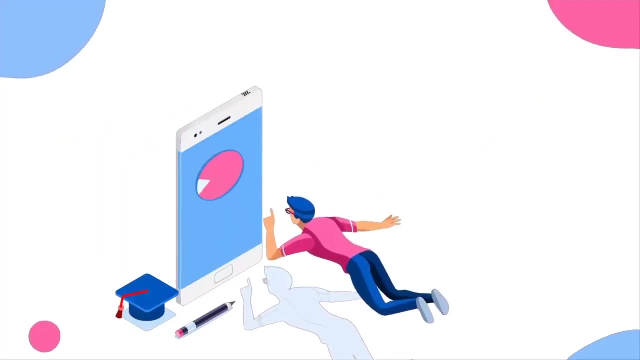 majority of the books are exam-oriented only. The focus is not on clearing the concepts, And hence it is very difficult for many students to understand the concepts clearly. But I have designed this course in such a way that every concept is unfolded at the right time. 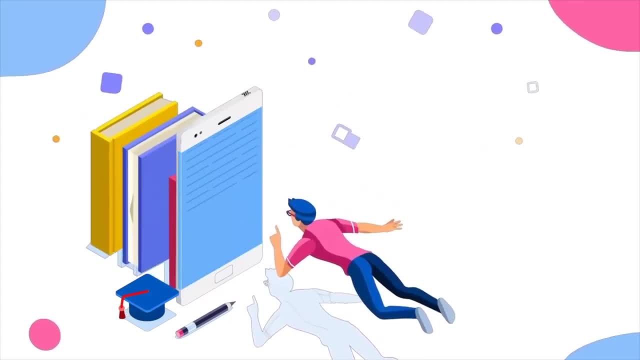 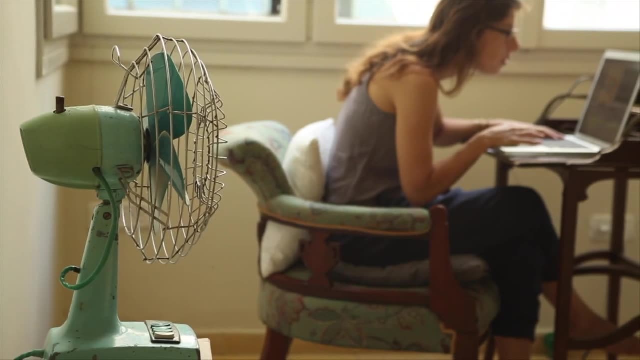 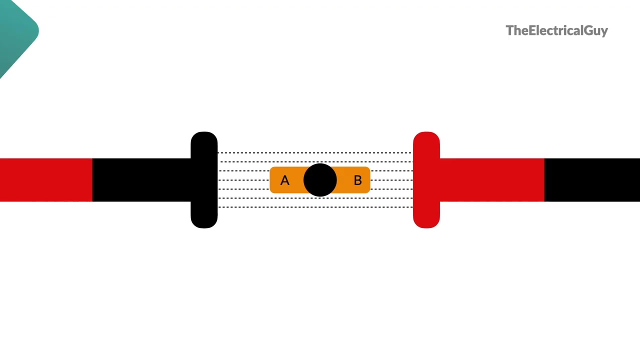 which makes the understanding very, very easy and interesting And you will not feel lost at any point of time. My main focus in this course is to clear the DC machines concepts first. Clearing the concepts is the primary goal of this course. In this course we will start our study by building a DC generator. 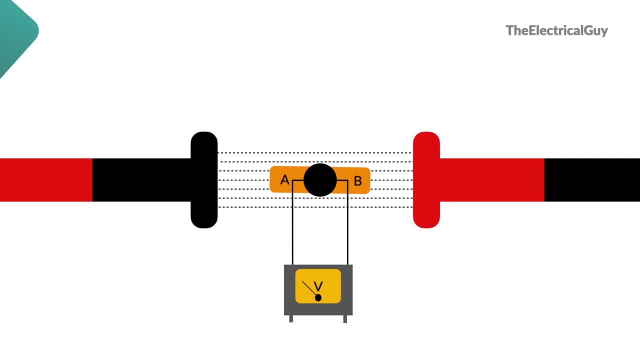 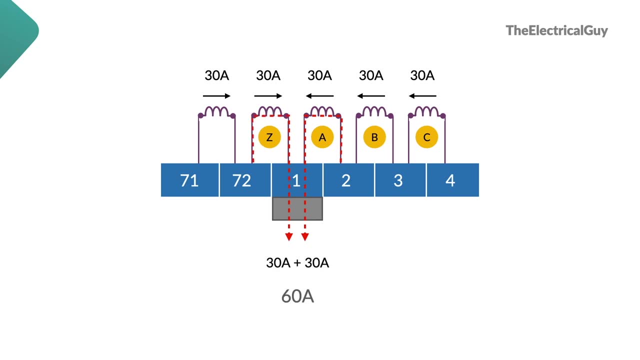 Of course virtually. Then we will understand how voltage is generated, what is armature reaction and its effect on our machine, what is commutation, what are the different types of DC generator and motor. We will also study their different characteristics and where we can use them. 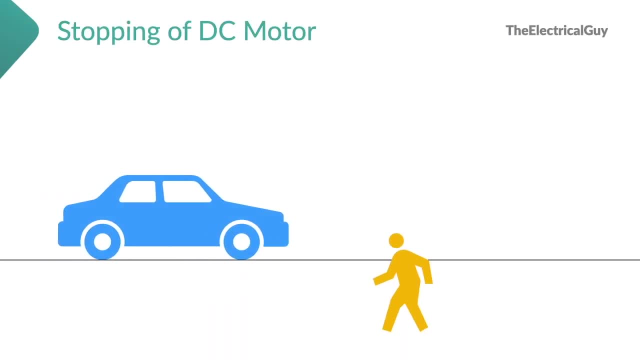 We will understand how we can control the speed of DC motor, how to apply brakes, different starters for motors, losses in DC machine and all the other things. The videos will be short and crisp And to the point, with no unnecessary talking. 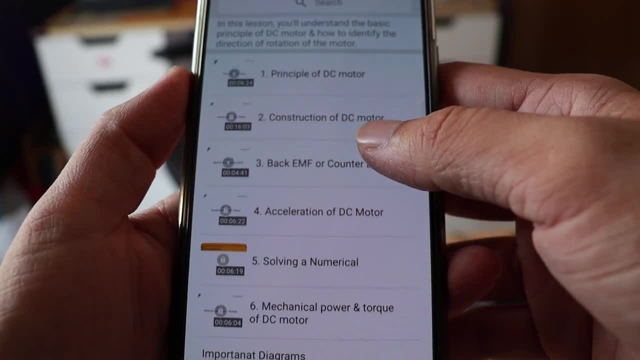 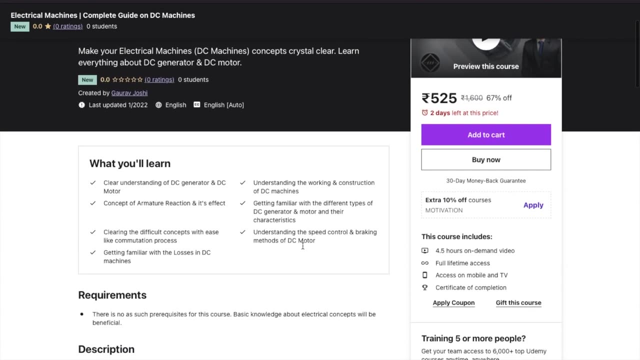 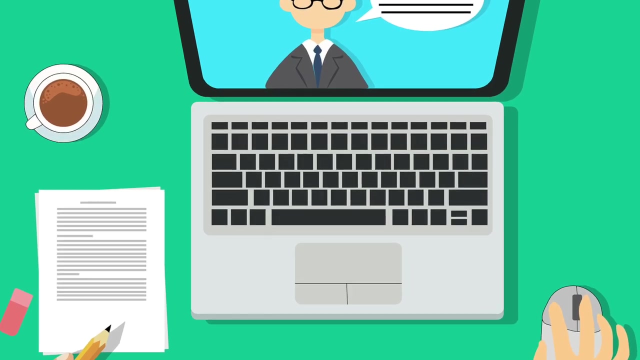 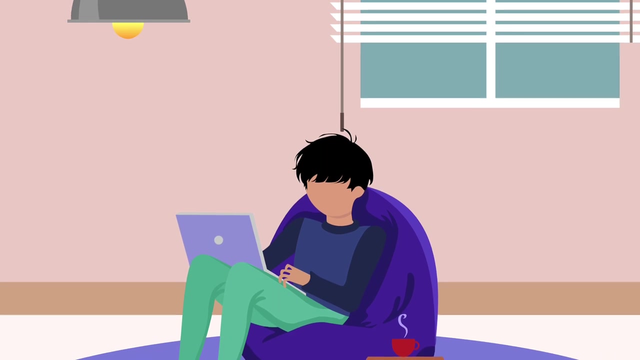 The course is available on the electrical guy mobile app. You can also join the course using Udemy. I will give link for both the options down in the description. Well, I am very much excited to take you through this exciting journey of understanding the DC machines. I am 100% sure that you will be learning a lot from this course and you are gonna. develop your ideas and your knowledge about the DC machines. I hope you will take this course with you. Thanks for your interest in electrical machine.